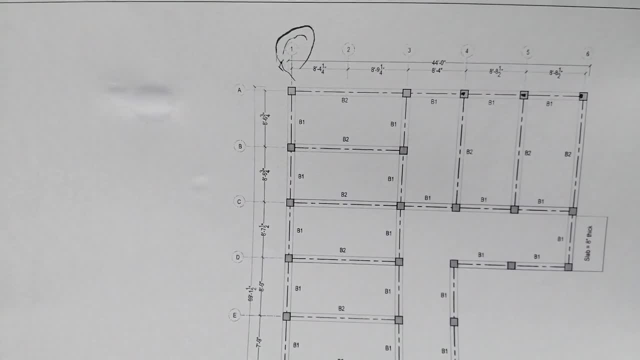 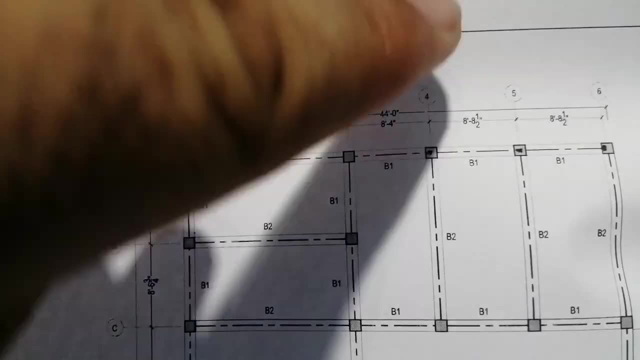 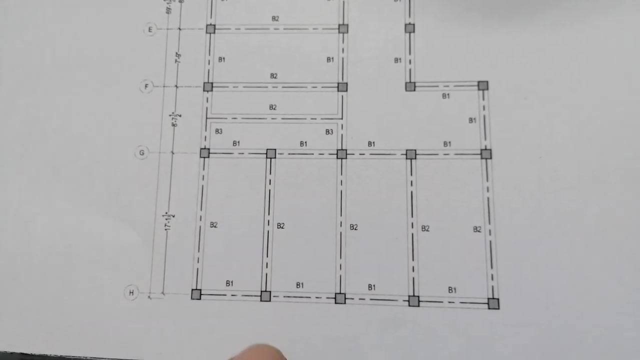 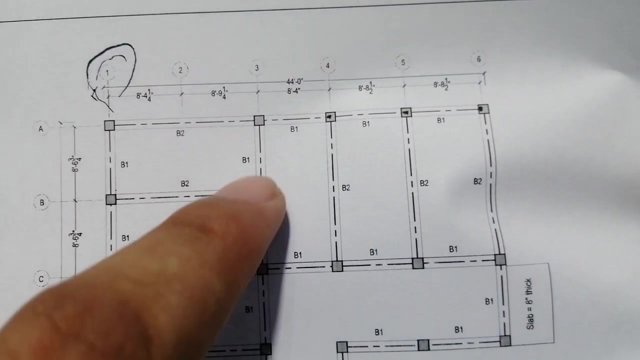 Which is column number one, Eight columns in column number one. we have, Second, we have the two, but we don't have the column here. As you can see, guys, this is two but we don't have column. Okay, So the column is coming here. as you can see, guys, this one One is this one. This is the second one column. Okay. Next, guys, you can see column three. It can show the. the dotted lines can show you the grade line for the columns. Okay, As you can see, these are. 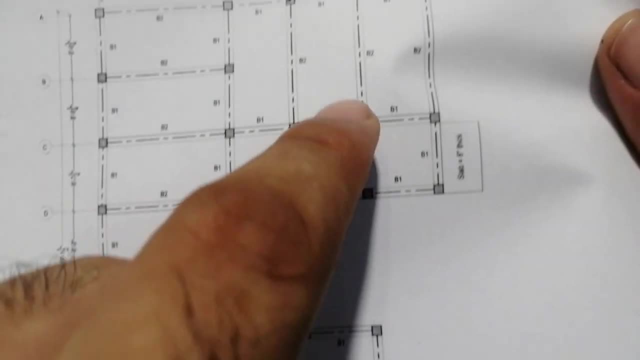 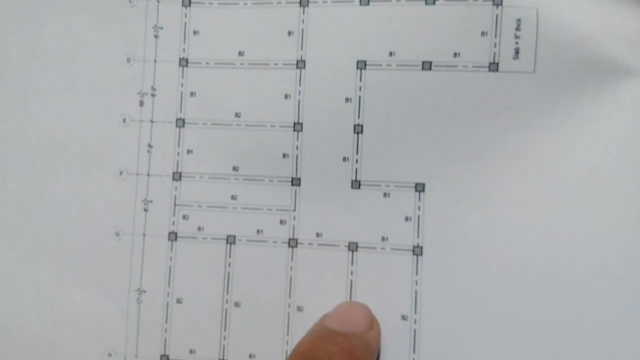 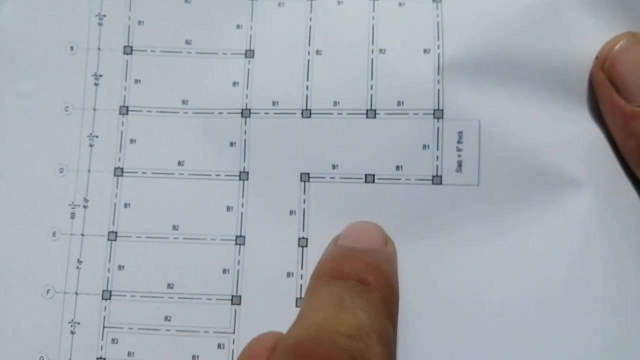 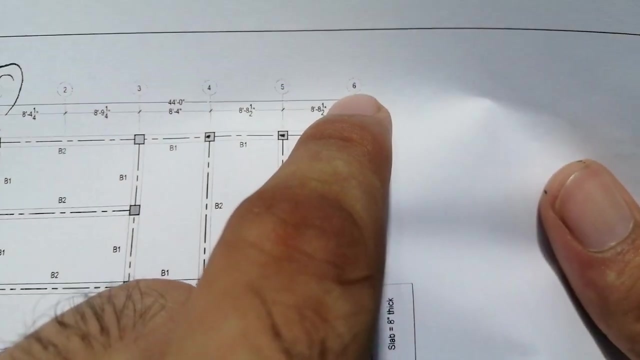 column three To this. Okay. Next guys, you can see column Column four. Okay, So this is four. So column four is here like this to this point. Next guys, you can see column five. Okay, So come from here. as you can see, we have three numbers: one, two, three columns- Sorry, Four, five, also six columns And column six. we have one, two, three. Next we are coming here. we don't have the other columns. 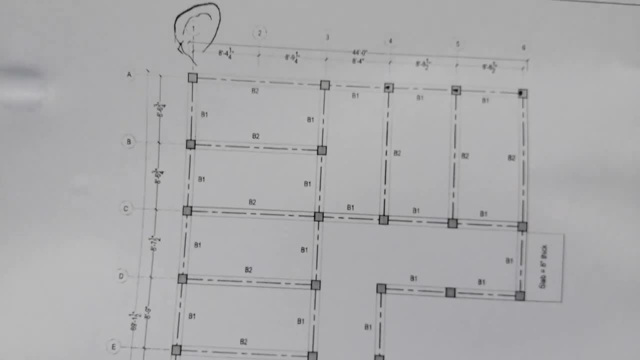 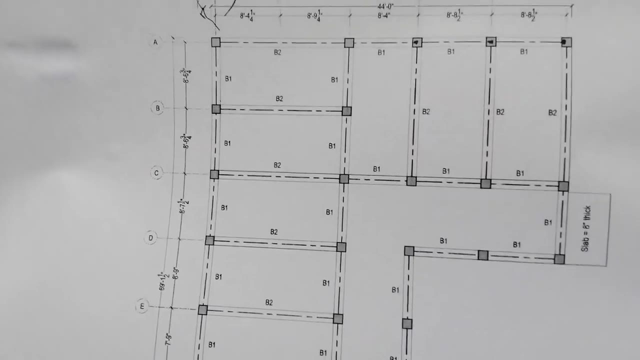 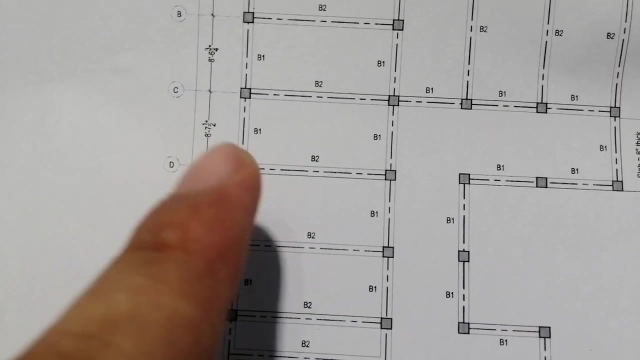 column: okay, so this can show you the grades of column. okay, column grades. the dotted line is the center line for this. next guys you can see- sorry for this next guys. you can see the b1 and b2 anywhere you can see. for the beam, beam 1 and beam 2. it means here, guys, the long beam is called b2. 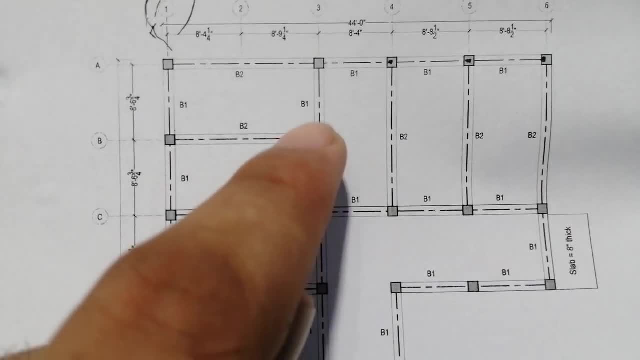 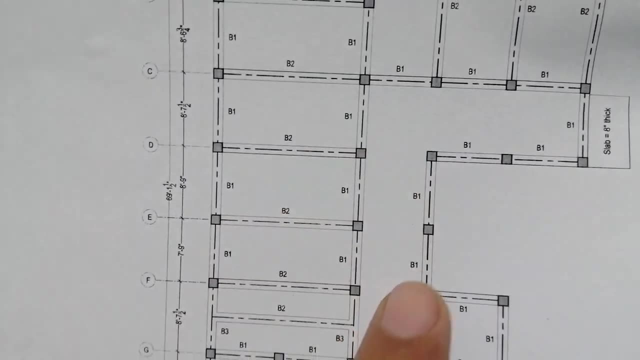 and the short beams are called b1, as you can see, b1, b1, b1, b2. long columns are b2, here b2, b2, b2. okay, so these are b1 and b2. p call, or so how you can read what is the specification of b1 and what is. 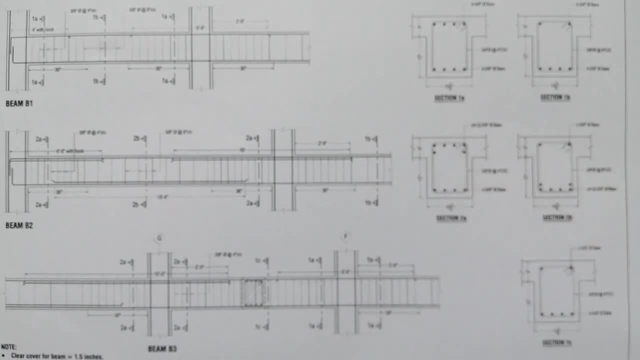 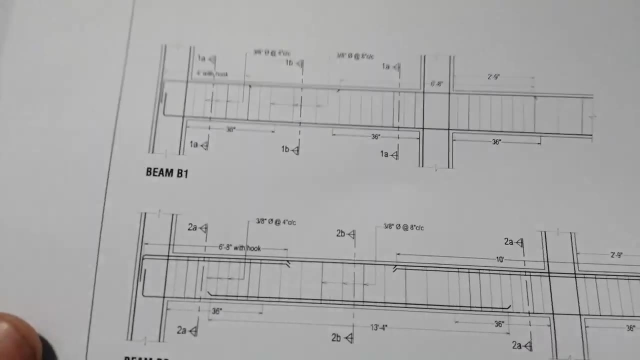 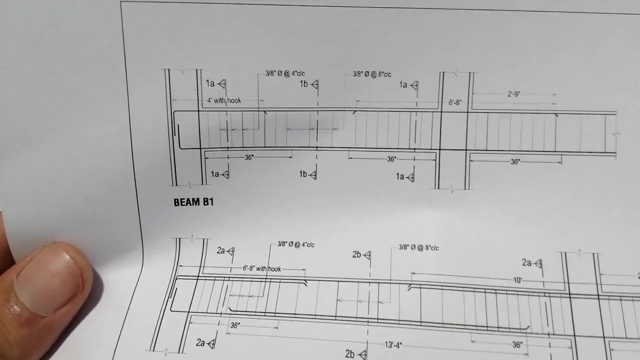 the specification of b2. next next, guys, you can see, this is the drawing for different beams, as i told you, b1 and b2. so here, guys, you can see, this is b1, guys, look here. okay, so this is b1. so, guys, this is the long section of b1. and here, guys, you can see: 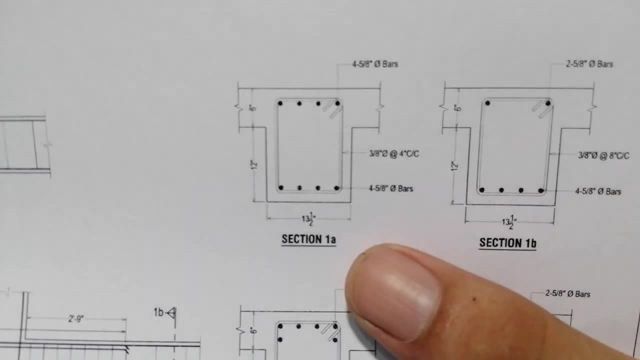 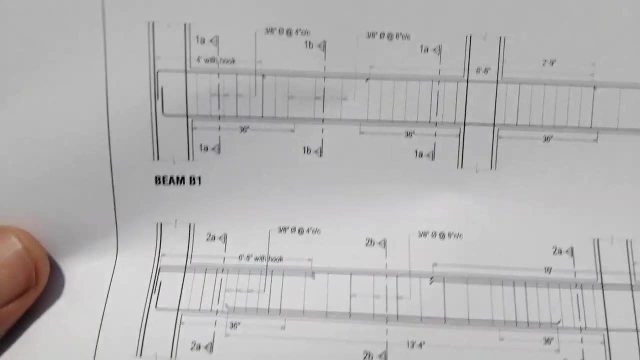 b1 and b2. so this is the long section of b1 and here, guys, you can see the long section of b1 and this is the section of b1. okay, and section a1 and section a- b, as you can see like this. okay, so for this you will check. okay, so b2, this is long column, guys, you can see b2, as i told you here. 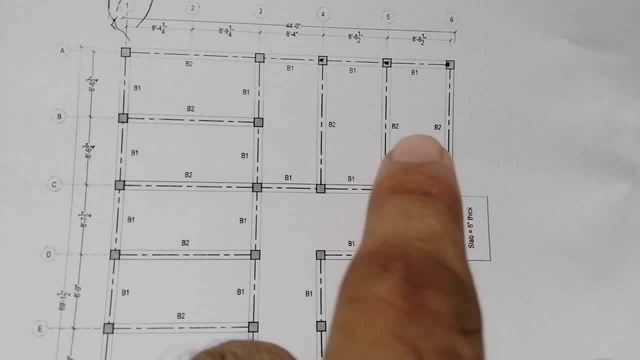 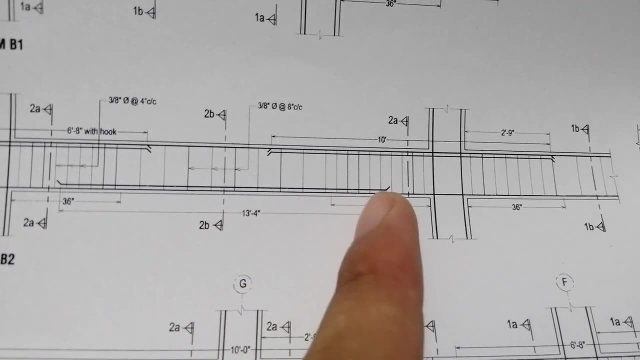 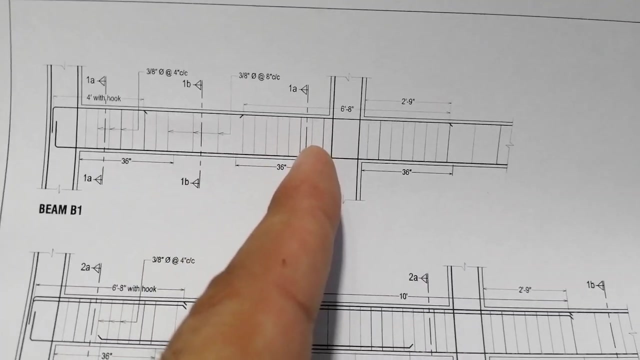 as you can see here, these are b2, b2 columns. okay, so x long section is this one. so you will check the specification of b2. what are here? as you can see, these are x reinforcement. so this is change. this beam b2, b1 is change. b1 is change from the b2. it's reinforcement detail is change. 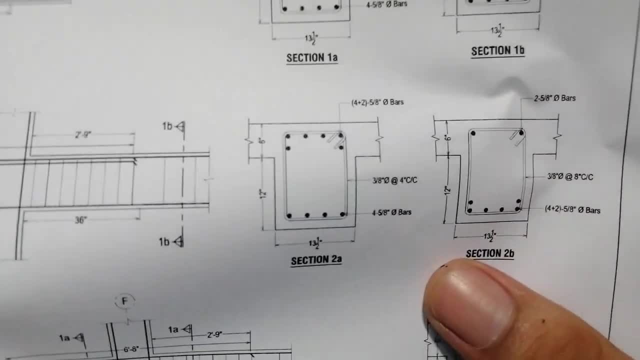 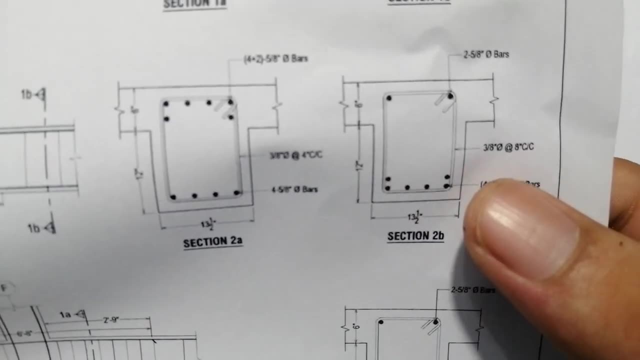 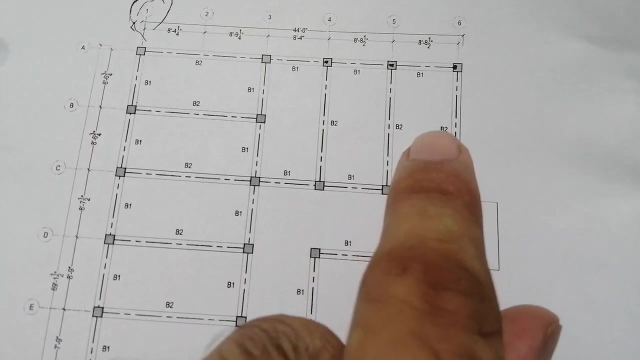 from this one. and also you can see guys at sections: okay, reinforcement details. look here. this is change from this one. okay, so now you can find what is the die of steel bar for top and bottom, etc. with the help of this. when you see this one so directly, you will come to this drawing and 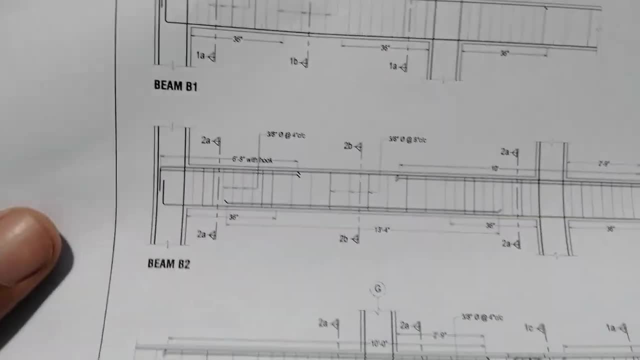 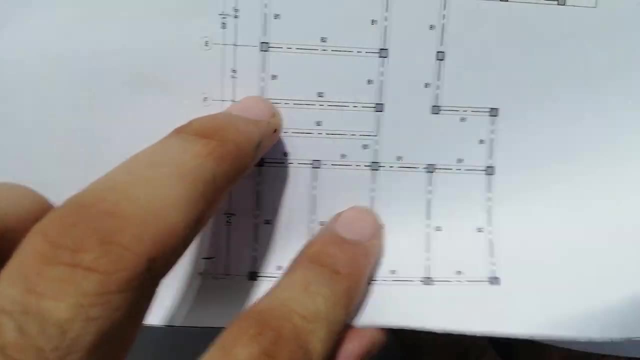 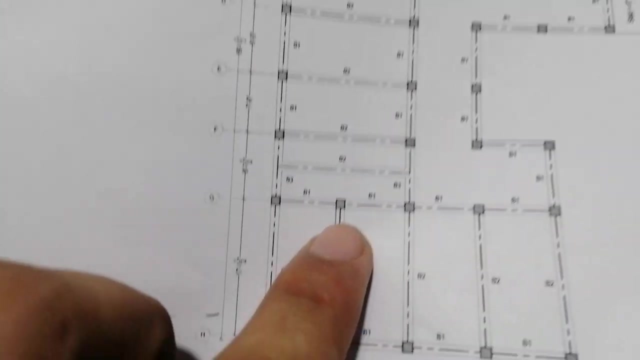 you will check b1 and b2 drawing its specification reinforcement details. now, guys, you can see this is b3, but here we don't have b3, so therefore we don't need to touch the b3. so if we have the b3 here, okay, then we will discuss. 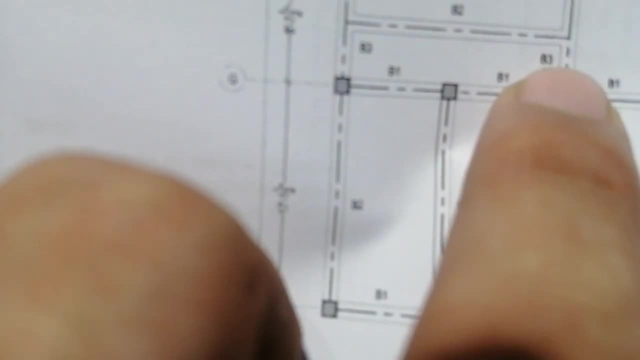 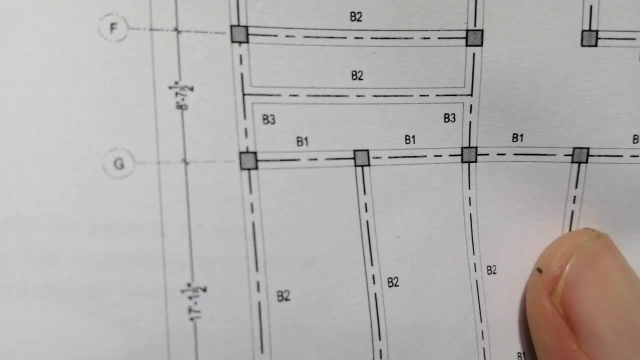 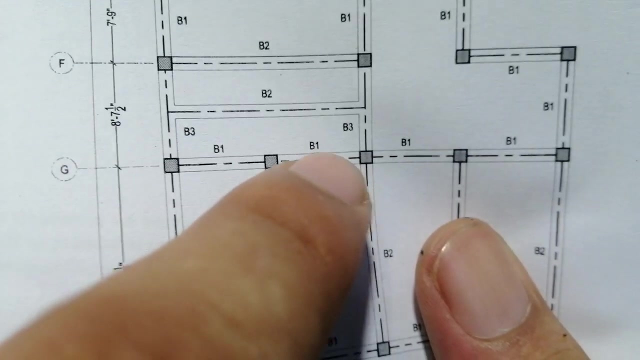 okay, here, guys, you can see this is b3. let me focus the camera. here, guys, you can see b3. we have. i was thinking that i don't have the b3. look here, this is b3. this is also b3. so for b3, for b3 beam, you will check this one. 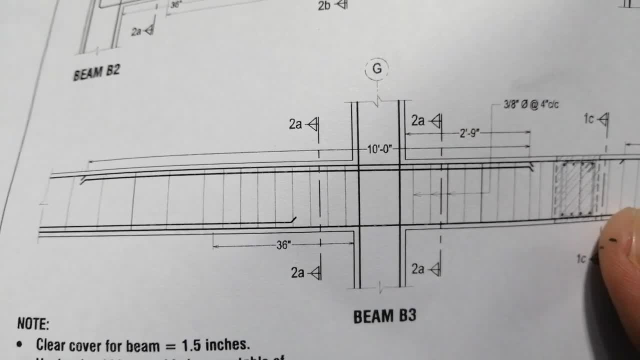 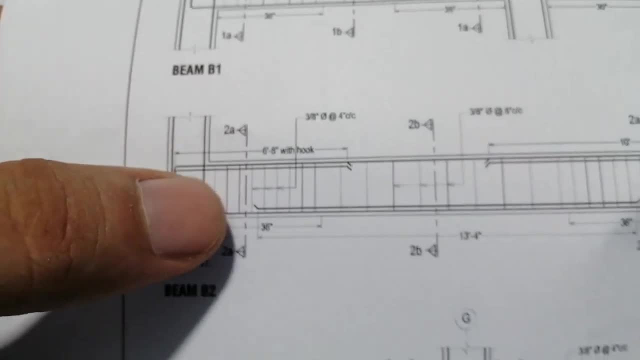 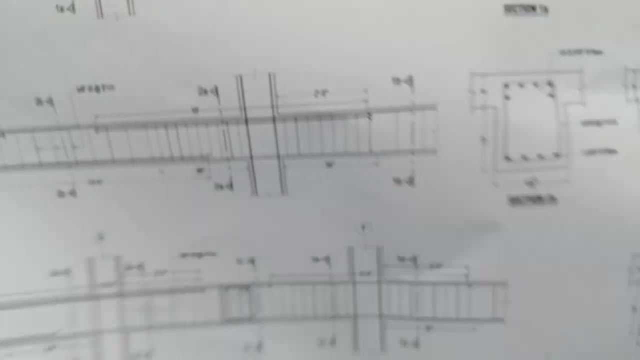 okay, this is x reinforcement details for b3, beam number three. look here: x reinforcement detail is changed from the b2 beam 2 and beam 2 is changed from the b1. okay, so x reinforcement at sections x section. you can see, guys, this is the section. 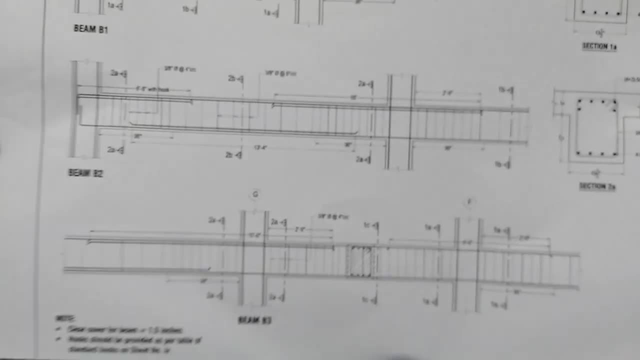 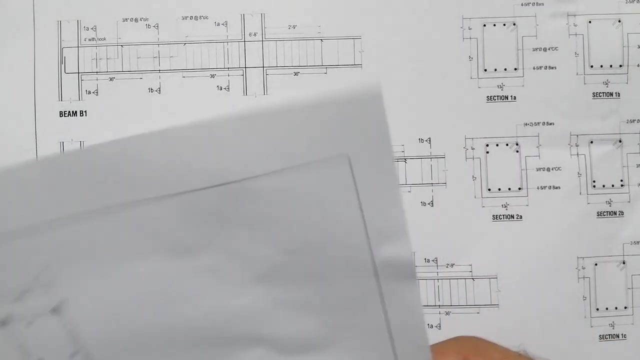 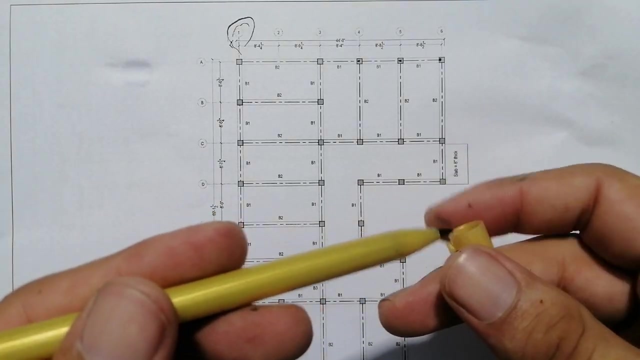 this one, okay. so, guys, this is a short video to discuss how to read engineering trying. so i will discuss its reinforcement detail. uh, if i have a time, so in next video i will. so this is just the way how to read seven engineering drawing, specially for building. so, guys, if you need, 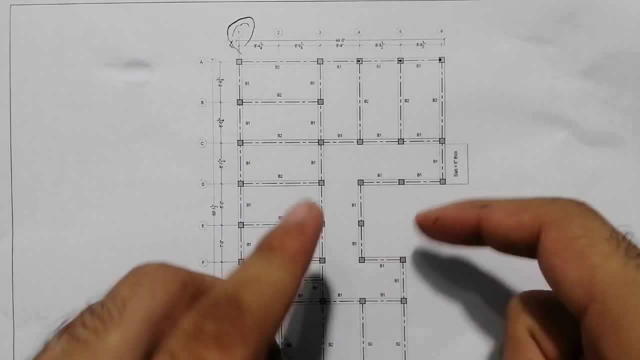 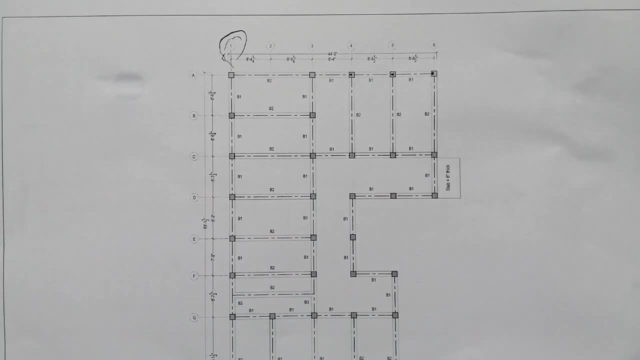 structural drawing, 2d, 3d, animation, etc. so you can contact me on this whatsapp number. i can do the best design for your house. thanks for watching. see you in next video. goodbye.